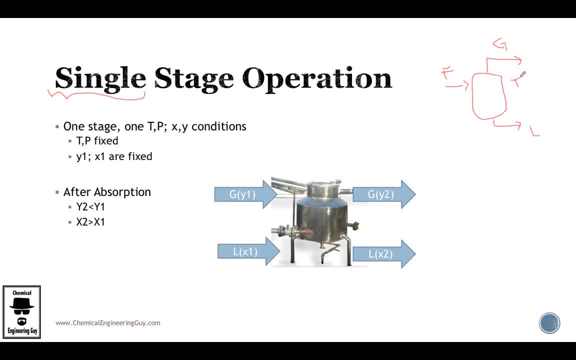 them into gas and liquid, because the flash has equilibrium conditions at the given temperature and pressures. so the same is true for absorption. remember that the main goal of absorption is to you have a gas with a solid, let's say Y will interact and with the liquid, and the liquid will strip, or the gas will. 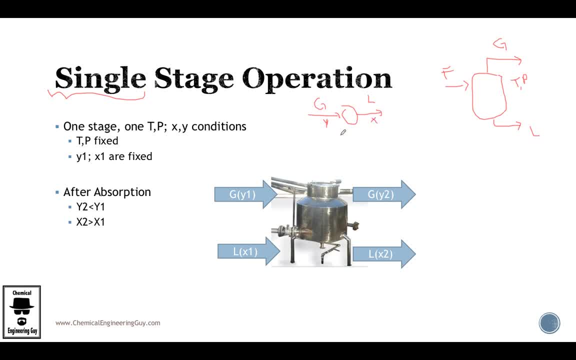 give the salt right here. let's call it X. used to differ the solute in the gas and liquid fraction phases. okay, so what are we saying here is that temperature and pressure will be fixed and the temperature and pressure will be, And if we have fixed condition or initial conditions, let's say 1, so at time 0, which technically is not time 0, but I like to say time 0.. 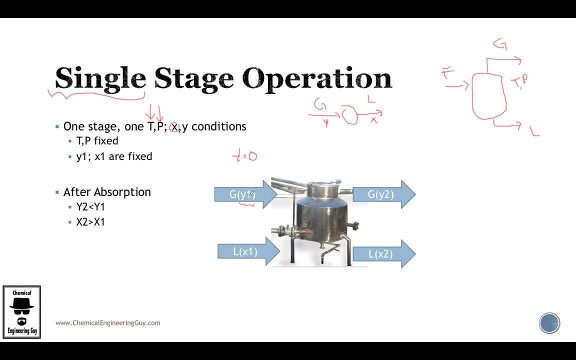 At the initial condition you will have a certain value of y1 at the gas phase. Let's say this is 3% of whatever material we're talking about. The main idea is to we know that the liquid has certain solubility towards this. 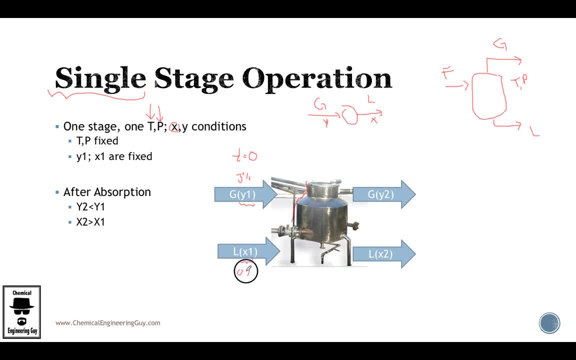 Let's say, initially this is 0, because this is pure, even though later on you can see that maybe it has 1%. so 3% and 1%, there's a little bit of interaction as well. So we have this part right here. let's say it's the tank or a container. 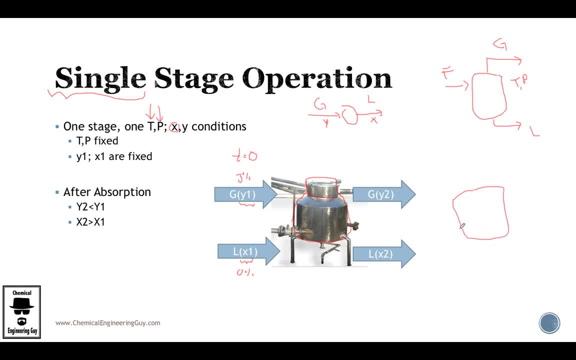 Actually, this is our system, the container, and we know that the liquid will be here and the gas will be here. So if we let this to enter in equilibriums, let's say y Fraction, y1, and x1.. 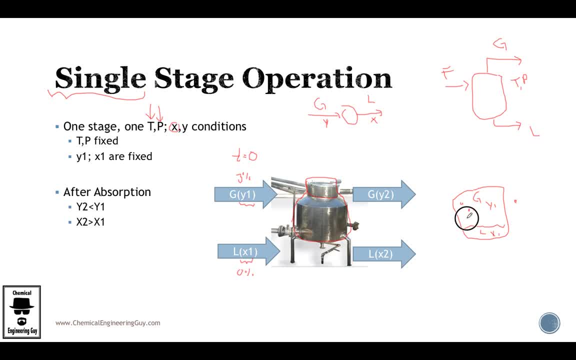 We know that the solute- let's let it be these little guys- dots, So they will go to liquid phase because of equilibrium. Remember that you need to choose or select a solvent that favors this. If you know that the liquid you're using does not favor this, then you fail at the selection of the solvent. 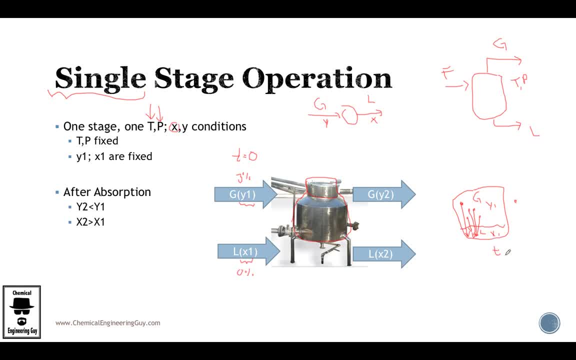 So this: we let time pass, and let's say, time passes by and this is now time x. Well, actually, let's use time after. let's say: this is time B. So this is initially, and this is time B, which is when equilibrium is achieved. 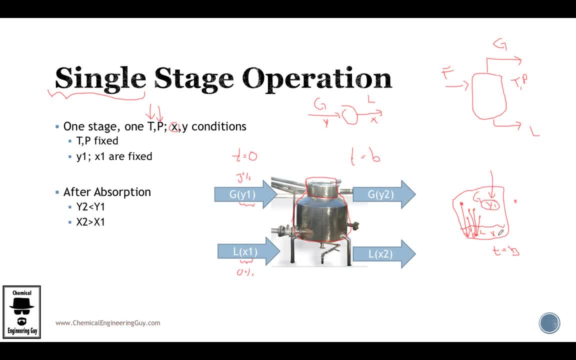 So we know that not any longer. y1 is the same value and x1, by definition, can't be the same number, So let's call this after this time: y2 and the liquid x2.. So we know that this will decrease because 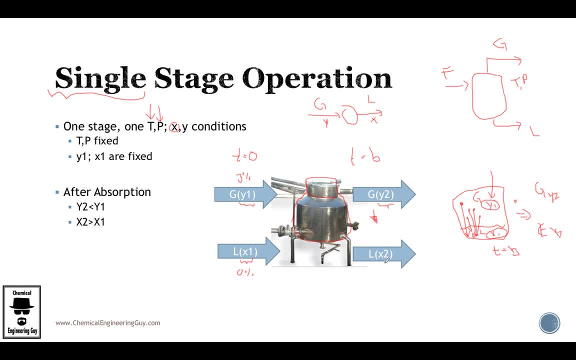 material has gone to the liquid phase and this must increase. so we have here, we know, that the gas is getting leaner, or let's say it's getting clean, and the liquid is stripping the salt, so it must increase in concentration. so, as you can see, this will be a good absorption process. but what? what will happen if? 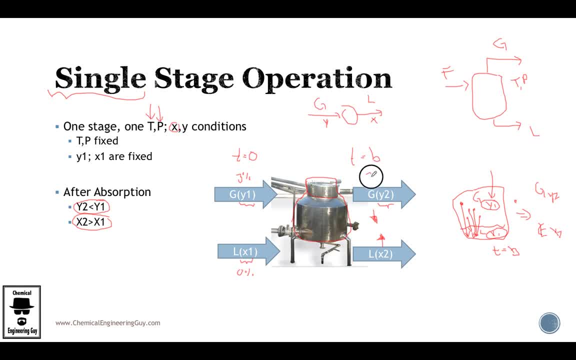 actually we want to remove three percent. let's say this was two percent and this went to one percent, and let's say that we want final conditions or maybe 0.5 percent in the gas phase. so of course there was another. let's say engineer, we 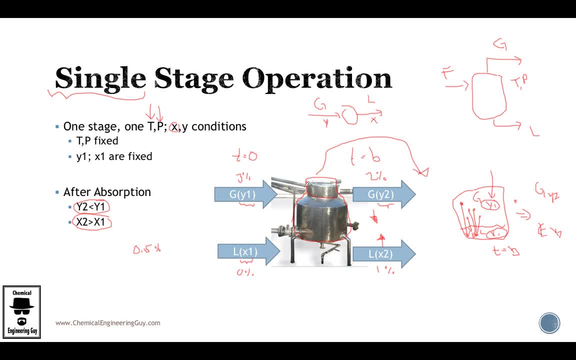 thought: why not add another extra stage? we can see that one percent decrease. let's see if we add another stage. let's see if we add another stage. let's see if we add another stage and maybe we decrease a little bit more so, and maybe we decrease a little bit more so. 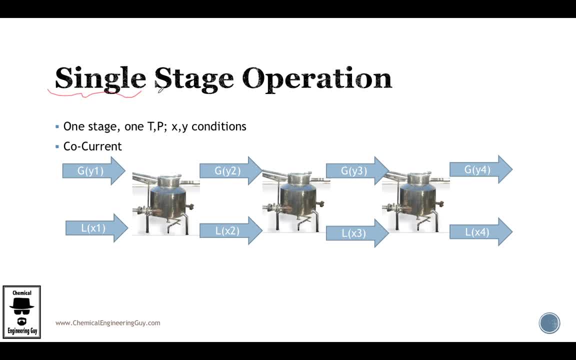 and maybe we decrease a little bit more. so this is the main idea of multiple. this is the main idea of multiple. this is the main idea of multiple stages. we are working with several stages. we are working with several stages. we are working with several single stages. so remember each of the. 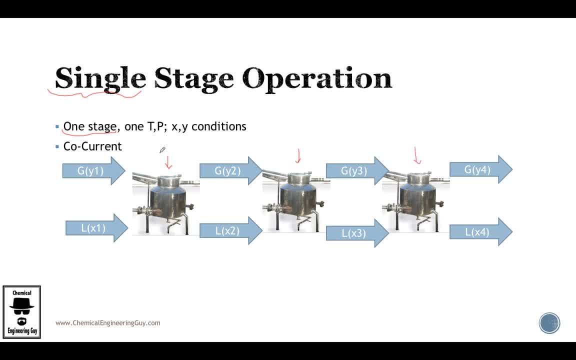 single stages. so remember each of the single stages. so remember each of the container is one stage. but what we are container is one stage, but what we are container is one stage. but what we are doing is arranging these in several. doing is arranging these in several. doing is arranging these in several stages, so all of them have the same. 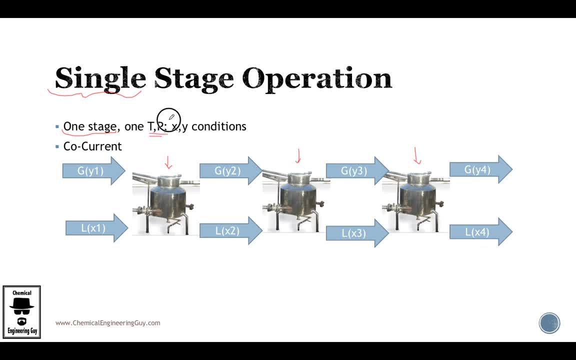 stages. so all of them have the same stages. so all of them have the same temperature and pressure conditions, but temperature and pressure conditions, but temperature and pressure conditions. but they do not have the same liquid and gas. they do not have the same liquid and gas. they do not have the same liquid and gas phase conditions. that is, y1, y2, y3 and 4. phase conditions, that is, y1, y2, y3 and 4. phase conditions, that is, y1, y2, y3 and 4, and X, 1, 2, 3 & 4 are not the same and X, 1, 2, 3 & 4 are not the same. 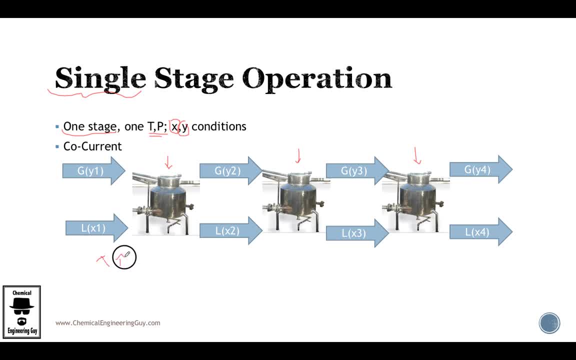 and X. 1, 2, 3 & 4 are not the same. actually, as you can see, X is going to. actually, as you can see, X is going to. actually, as you can see, X is going to increase as we follow to the right and Y. 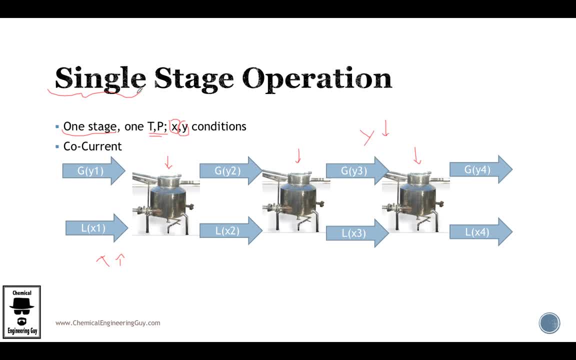 increase as we follow to the right, and Y increase as we follow to the right, and Y should decrease as we go to the right. should decrease as we go to the right. should decrease as we go to the right. okay, this type of operation is called. okay, this type of operation is called. 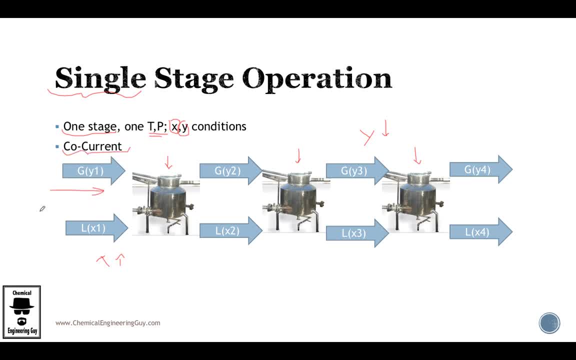 okay, this type of operation is called co-current flow. you can see the flows: co-current flow. you can see the flows- co-current flow. you can see the flows or the currents go in the same manner, so, or the currents go in the same manner, so, or the currents go in the same manner. so what happened here is maybe we got this. 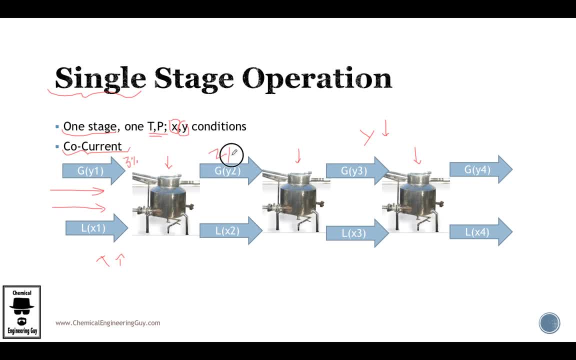 what happened here is: maybe we got this. what happened here is: maybe we got this: 3%, remember we were operating, and then 3%, remember we were operating, and then 3%- remember we were operating, and then we got 2% and then we got maybe a 1%. 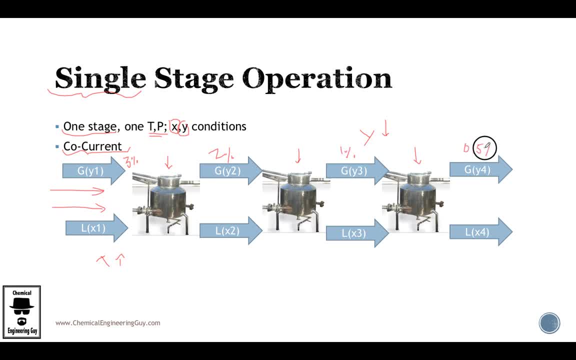 we got 2% and then we got maybe a 1%. we got 2% and then we got maybe a 1%, and remember that our objective was to, and remember that our objective was to, and remember that our objective was to get to 0.5%. so you can see, this is a. 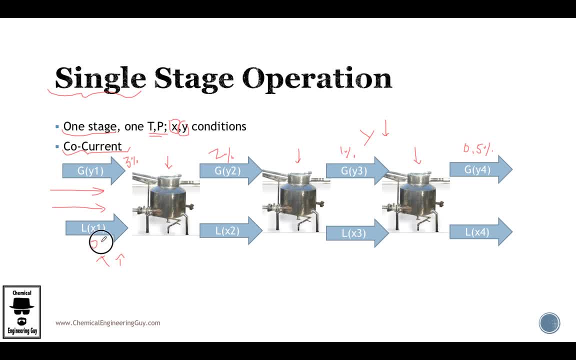 get to 0.5%. so you can see this is a get to 0.5%. so you can see, this is a very creative way to use stages and it very creative way to use stages and it very creative way to use stages. and it was 0%. maybe it increased to 1% and then 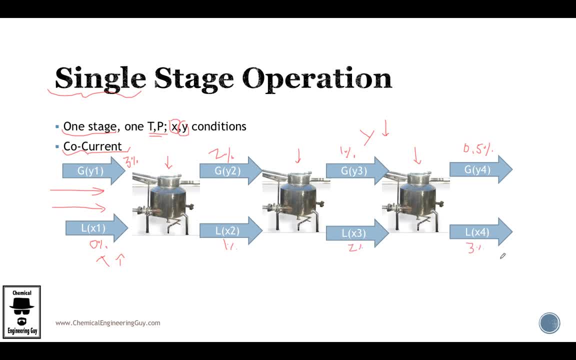 was 0%, maybe it increased to 1% and then was 0%, maybe it increased to 1% and then 2% and maybe even 3%. this will be what: 2% and maybe even 3%. this will be what. 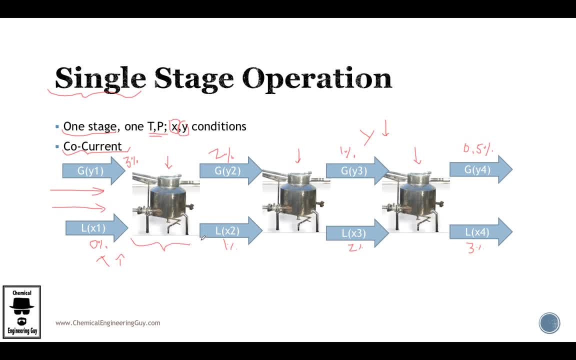 2% and maybe even 3%. this will be what you will want. but the problem right here, you will want, but the problem right here, you will want. but the problem right here is that it's kind of tedious to work. is that it's kind of tedious to work? 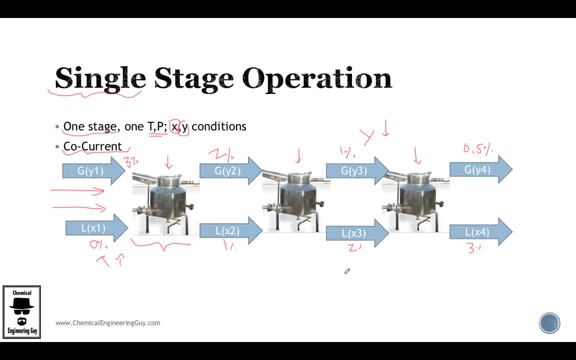 is that it's kind of tedious to work with several unit operations and, as you, with several unit operations and as you with several unit operations, and as you can see, they will take plenty of time. can see they will take plenty of time. can see they will take plenty of time because the construction is going to be. 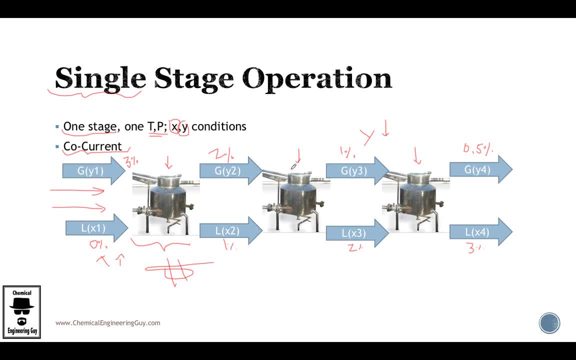 because the construction is going to be, because the construction is going to be expensive and it's kind of hard to have expensive and it's kind of hard to have expensive and it's kind of hard to have the same conditions- temperature- and the same conditions- temperature and. 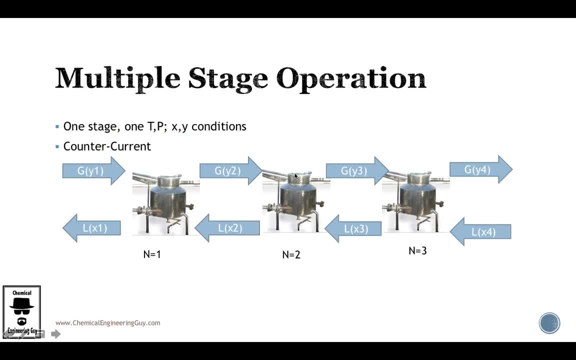 the same conditions: temperature and pressure, even though it will be great if pressure, even though it will be great if pressure, even though it will be great if we could do that. so another type of we could do that. so another type of we could do that. so another type of operation is the counter current. 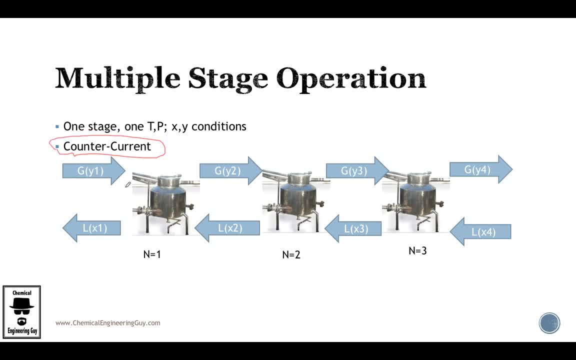 operation. is the counter current operation. is the counter current operation. we're going to see those later operation. we're going to see those later operation. we're going to see those later on. but this makes more sense in that on. but this makes more sense in that on. but this makes more sense in that this is very low. in this case, X will be. 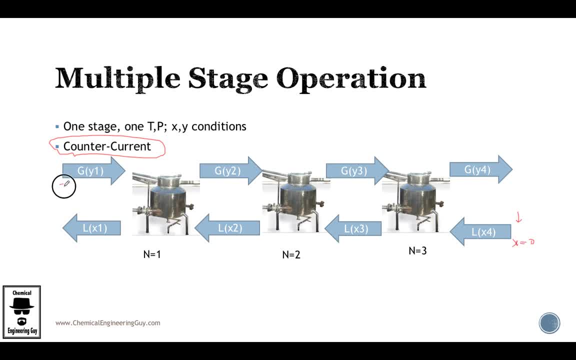 this is very low. in this case, X will be. this is very low. in this case, X will be 0 because it's the clean solvent, and the 0 because it's the clean solvent and the 0 because it's the clean solvent and the gas is the highest concentration, right? 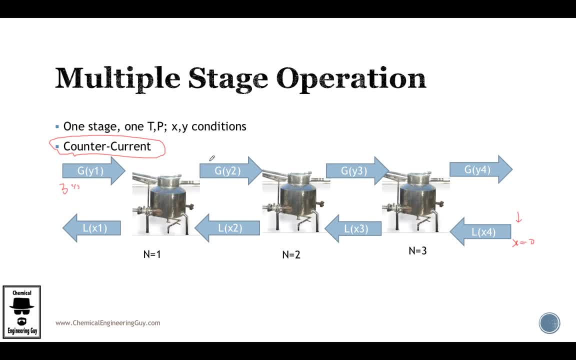 gas is the highest concentration, right. gas is the highest concentration right here in the initial condition. so what's here in the initial condition? so what's here in the initial condition? so what's happening here is that 3 decreases to 2. happening here is that 3 decreases to 2. 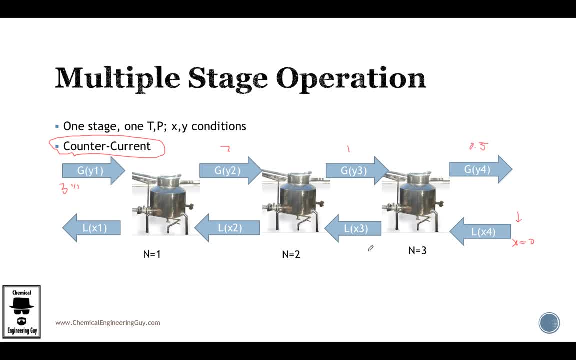 happening here is that 3 decreases to 2, 1 and 0.5, and still these go. 1, 2 & 3, 1 and 0.5, and still these go. 1, 2 & 3, 1 and 0.5, and still these go 1, 2 & 3. the main difference is that when we 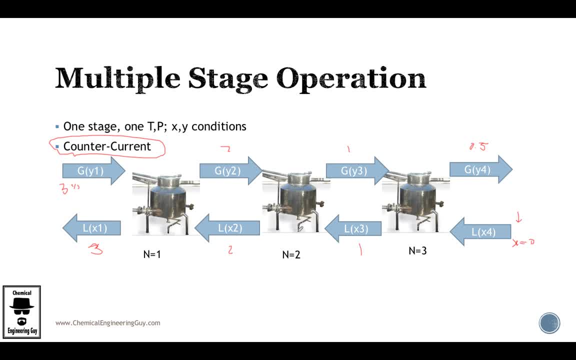 the main difference is that when we- the main difference is that when we design, we will see that this takes less design. we will see that this takes less design. we will see that this takes less time and it's much more efficient. we're time and it's much more efficient we're. 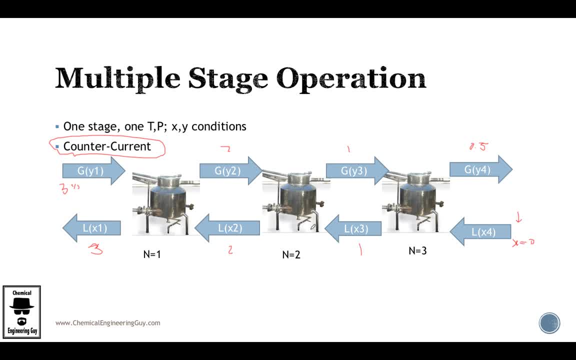 time and it's much more efficient. we're going to explain that later on, but what going to explain that later on? but what going to explain that later on? but what I want you to get the idea is that it's I want you to get. the idea is that it's. 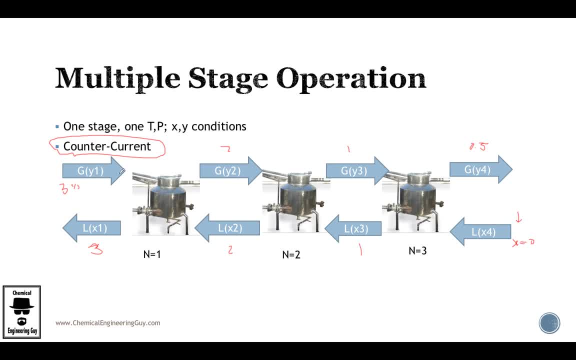 I want you to get the idea is that it's kind of hard to favor this condition, as kind of hard to favor this condition, as kind of hard to favor this condition as it goes because the liquid to the left, it goes because the liquid to the left. 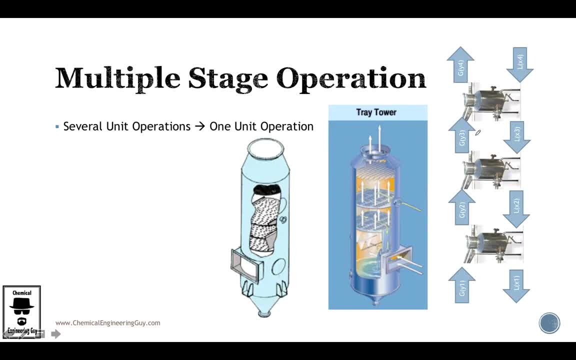 it goes because the liquid to the left, the gas to the right, so someone had the, the gas to the right, so someone had the, the gas to the right, so someone had the brilliant idea to build a tower with brilliant idea to build a tower, with brilliant idea to build a tower with several, let's say, stages. because we 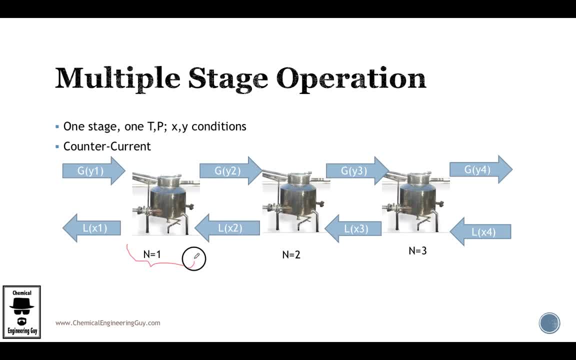 several, let's say stages, because we several, let's say stages, because we already, as you can see, we're already already, as you can see, we're already already, as you can see, we're already working with multiple stages. this is working with multiple stages, this is working with multiple stages. this is stage number one, stage, number two, stage. 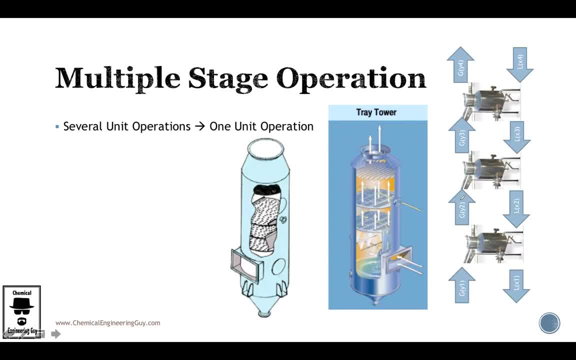 stage number one. stage number two. stage stage number one. stage number two. stage number three. so what? someone another number three? so what? someone another number three? so what someone another engineer imagine was what if I build a engineer imagine was what if I build a engineer imagine, was what if I build a tower instead of a pipe? even though you 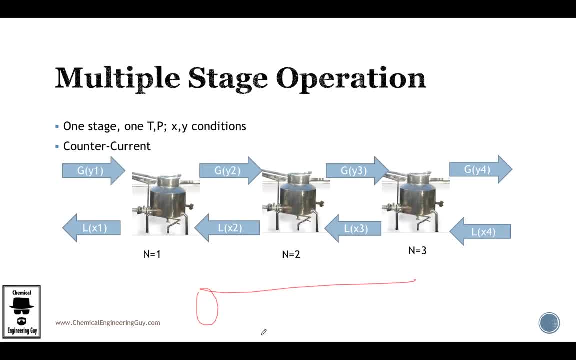 tower instead of a pipe. even though you tower instead of a pipe, even though you could in theory make this arrangement, could in theory make this arrangement, could in theory make this arrangement- maybe a pipe with several trays, but maybe a pipe with several trays, but maybe a pipe with several trays, but actually what is much more efficient and 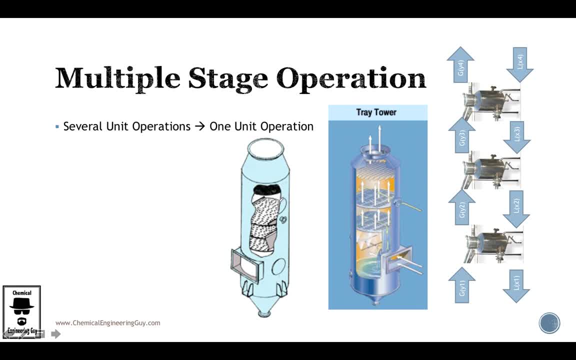 actually what is much more efficient, and actually what is much more efficient- and you will get to see that in the industry. you will get to see that in the industry. you will get to see that in the industry we see these extensively- is towers, so in, we see these extensively is towers, so in. 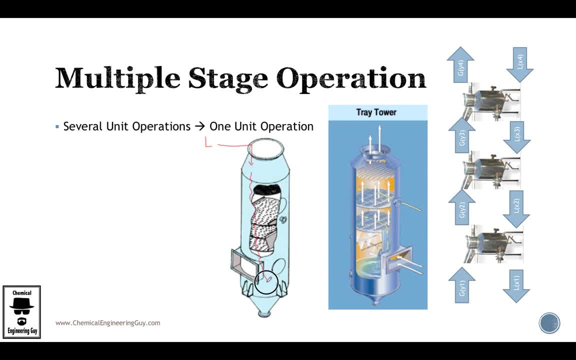 we see these extensively is towers. so in, here you get the liquid. you know that, here you get the liquid. you know that, here you get the liquid. you know that the liquid is going to drop by gravity. the liquid is going to drop by gravity, the liquid is going to drop by gravity and the gas goes directly. here you know. 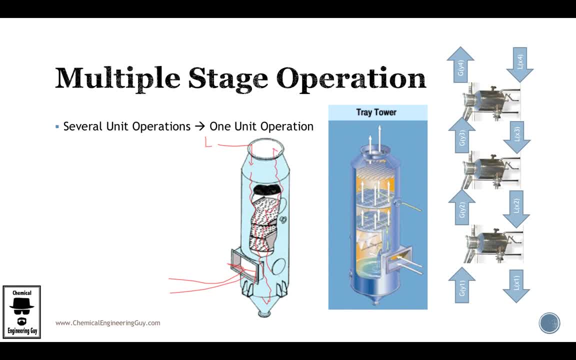 and the gas goes directly here. you know, and the gas goes directly here. you know that the gas, because it has difference, that the gas, because it has difference, that the gas, because it has difference in densities, will go upwards, it is in densities, will go upwards, it is. 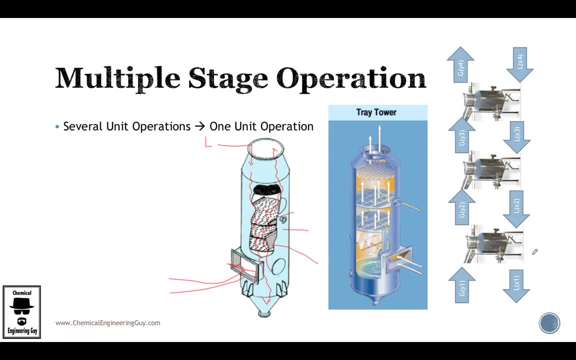 in densities will go upwards. it is exactly the same. we got here the trace. exactly the same. we got here the trace. exactly the same. we got here the trace tray 1, 2 & 3. so we've got tray 1, 2 & 3. 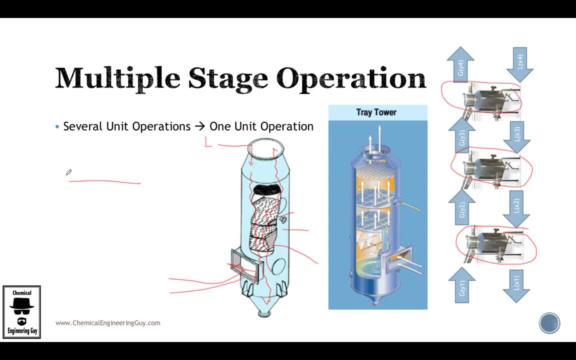 tray 1, 2 & 3, so we've got tray 1, 2 & 3. tray 1, 2 & 3, so we've got tray 1, 2 & 3. the main idea is that actually each tray. the main idea is that actually each tray. 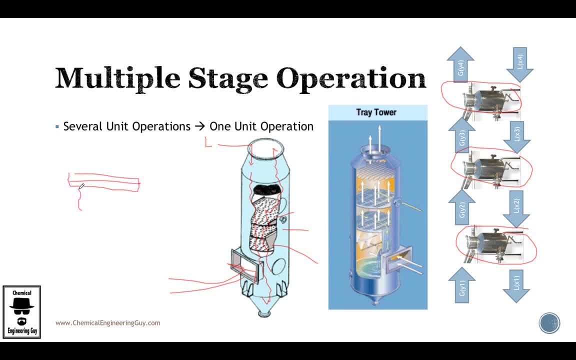 the main idea is that actually each tray can act as this unit operation and you can act as this unit operation and you can act as this unit operation and you will see that the trays are very much, will see that the trays are very much, will see that the trays are very much cheaper than the unit operation is. 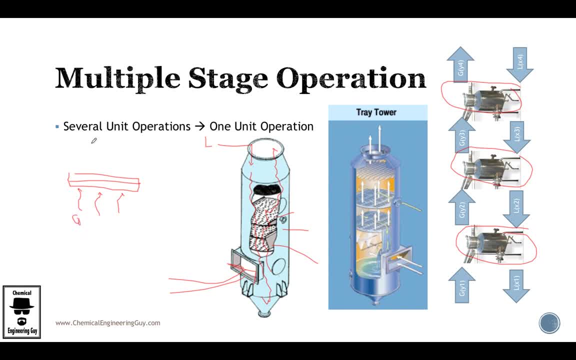 cheaper than the unit operation, is cheaper than the unit operation is it's separated. so the tray what favors? it's separated. so the tray what favors? it's separated. so the tray what favors? is that gas interacts with the liquid, is that gas interacts with the liquid, is that gas interacts with the liquid. so this is called multiple stage. 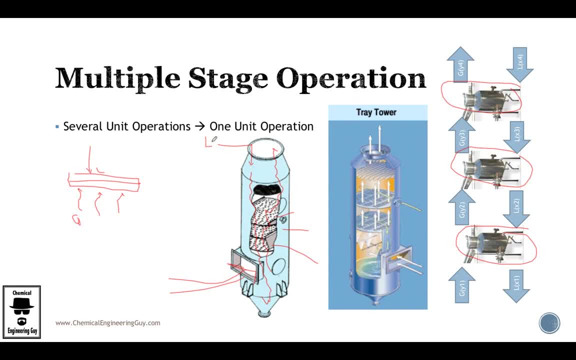 so this is called multiple stage. so this is called multiple stage operation. this is counter current operation. this is counter current operation. this is counter current operation. even though you could have a operation, even though you could have a operation, even though you could have a multiple stage operation, you could have. 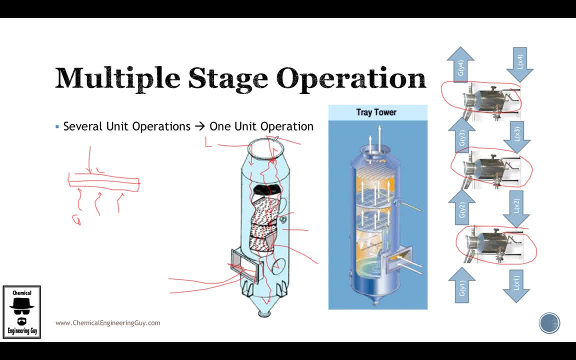 multiple stage operation. you could have multiple stage operation. you could have the addition of gas. even though it will the addition of gas, even though it will the addition of gas, even though it will be kind of hard to favor, you will have. be kind of hard to favor, you will have. 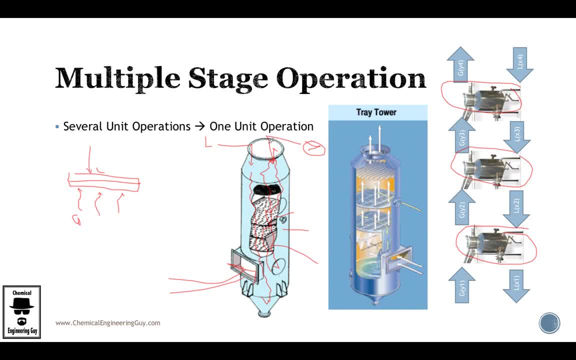 be kind of hard to favor. you will have to to to add much more compression here. you will to add much more compression here. you will to add much more compression here you will have arrangement: the counter current have arrangement. the counter current have arrangement, the counter current operation in vertical. 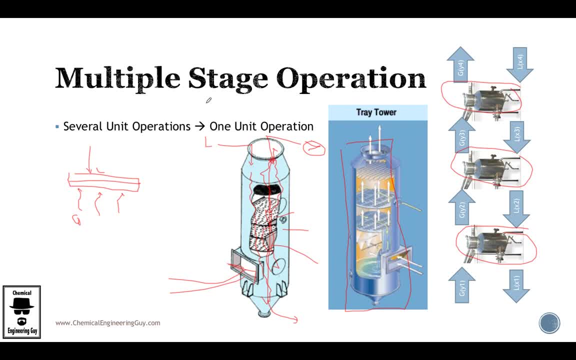 operation in vertical operation in vertical columns. okay, so hopefully you get the idea columns. okay, so hopefully you get the idea columns. okay, so hopefully you get the idea of what is a single, of what is a single, of what is a single stage. it's very important if you don't get 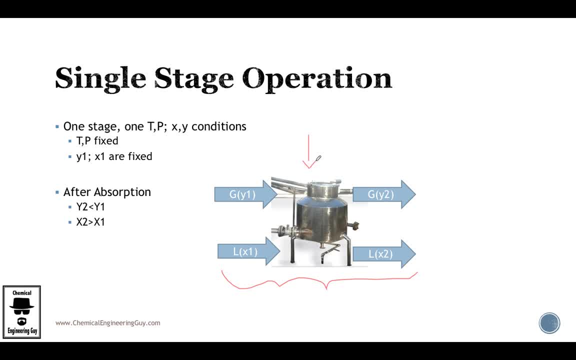 stage. it's very important if you don't get stage. it's very important if you don't get the idea of how absorption works in a, the idea of how absorption works in a, the idea of how absorption works in a single stage, single stage, single stage, while getting the idea of how it works. 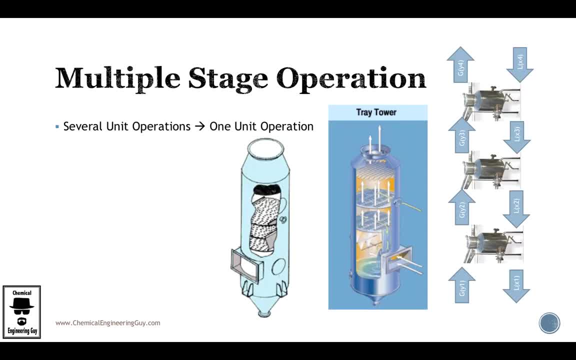 while getting the idea of how it works, while getting the idea of how it works in multiple stage counter current. in multiple stage counter current, in multiple stage counter current. concurrent flows, concurrent flows, concurrent flows. will be kind of hard, so please try to. will be kind of hard, so please try to. 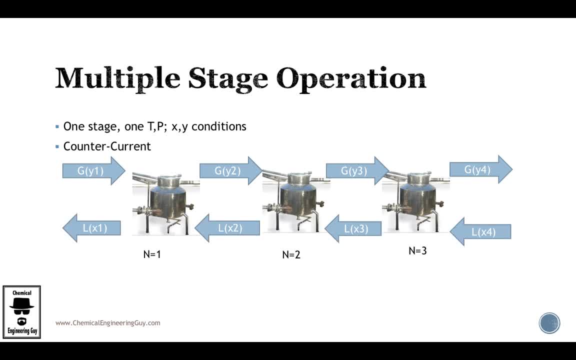 will be kind of hard. so please try to re, re, re review this section right here, this lecture, review this section right here, this lecture, review this section right here, this lecture, and understand why do we want several and understand why do we want several and understand why do we want several stages.